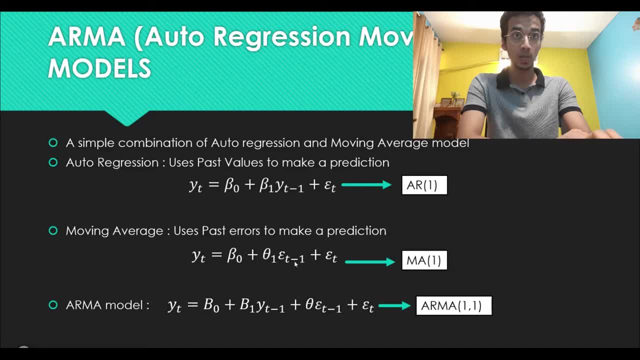 error in the previous time step, which is t minus 1 plus some error which you want to make in the current prediction Right. So very simple. Both of these things are going to work. Both of these models: they use the, one uses the pass value, one use the pass error. 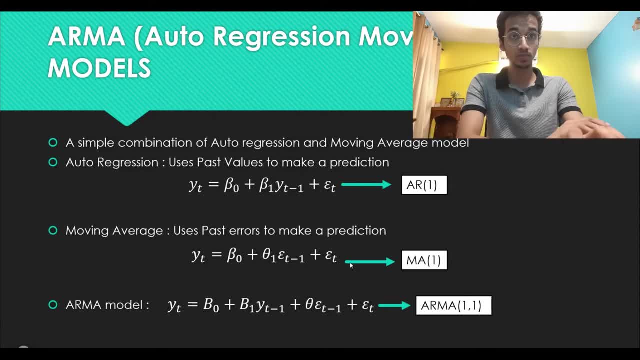 And since we're only using the values and errors from just the previous time step, these are called the order regression of order one and moving average of order one respectively, which is denoted by the one written over here in the bracket. So our model is simply a combination. 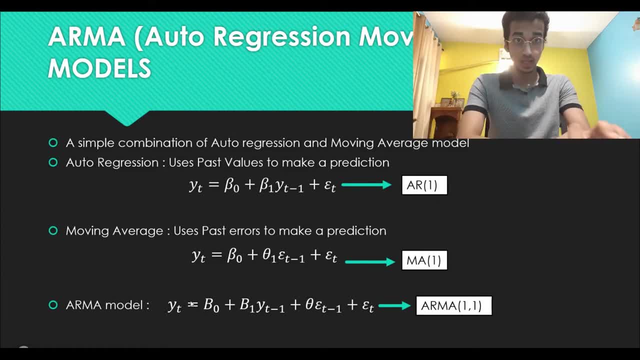 of both of these. So the equation for it would look like y sub t is equal to beta naught plus theta 1 into error made in the previous time step And error plus beta 1 into the past value plus some error which you want to make in. 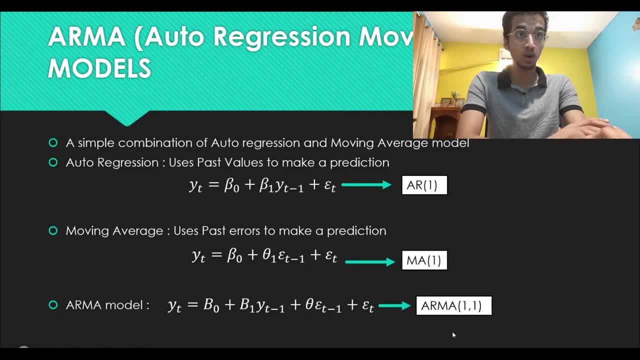 the current time step And it is represented as simply ARMA: one comma one right, So one represents. so one comma one basically represents that we're using auto regression of first order and moving average of first order, So it can be of different orders as well. you. 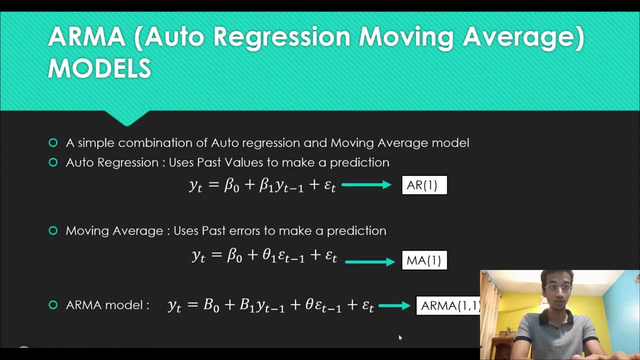 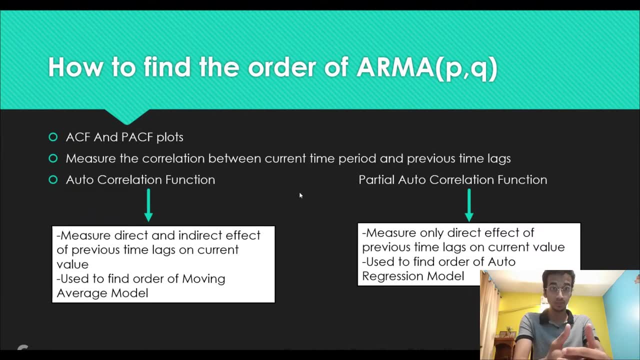 can use a different order of auto regression or a different order of moving average, which would look like this: it would have the notation ARMA p, comma q right, And question is: how do we find the order Right? How do we know if we should measure? 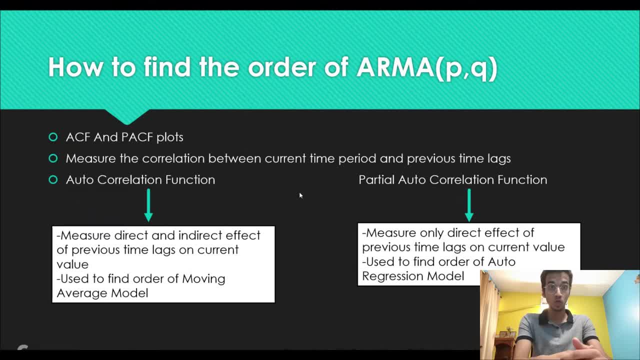 the value in the previous time step or two time steps back, Or should we check the error in two to three times this back? For that we use the ACF and PACF plots, which I have explained in their respective videos, But still, it's simply used to measure the correlation. 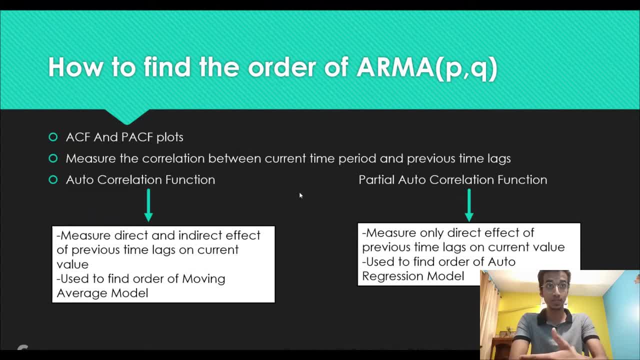 between the value of today and the value of some previous time steps back. So we have the auto correlation, partial auto correlation. Auto correlation simply measures the direct and indirect values of the order. So we have the order of the order and then we have the. 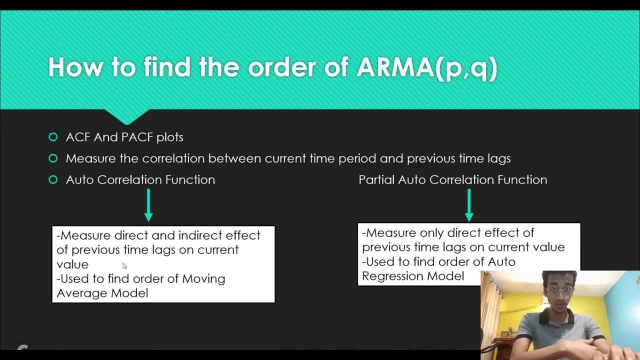 indirect effects of previous time lags on the current value And it is used to find the order of the moving average model And partial auto correlation measures. only the direct effect of the previous time lags on the current value. it eliminates the indirect effects And it is used to find the order of the auto regression model Right. So when? 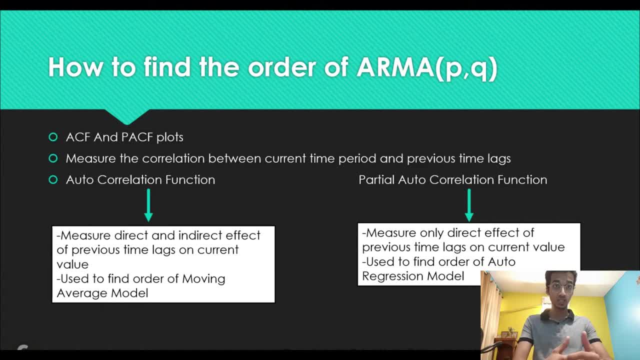 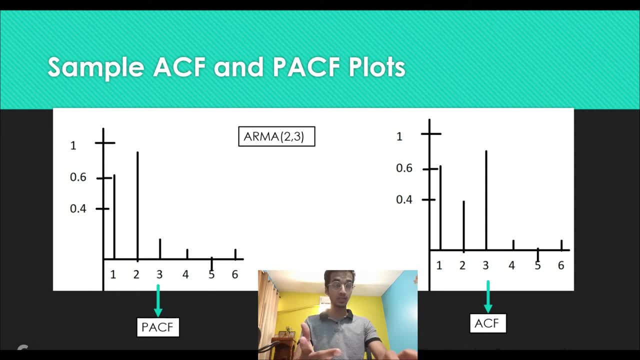 you have a time series and your first step should be to plot the ACF and PACF model. So let's say you get a plot something like this: On the left hand side we have the PACF plot And on the right hand side we have the ACF. 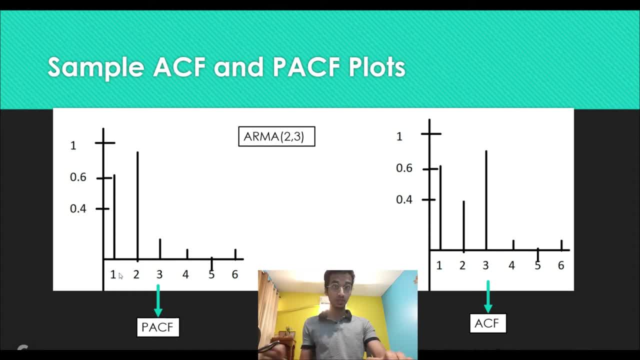 plot. On the x axis you have the time periods right. One basically means one time period back, two means two time periods back, and so on. And on the y axis you have the correlation, which is a value between minus one to one if you're using the Pearson correlation coefficient. 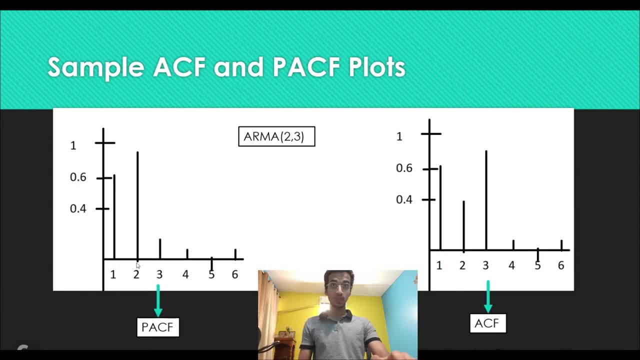 right. So you can see that for values one and two we have high values of correlation, which is 0.6 and something around 0.8, which means the first and second time period lags are relevant And the PACF will tell you the order of the auto regression model. So you can see that. 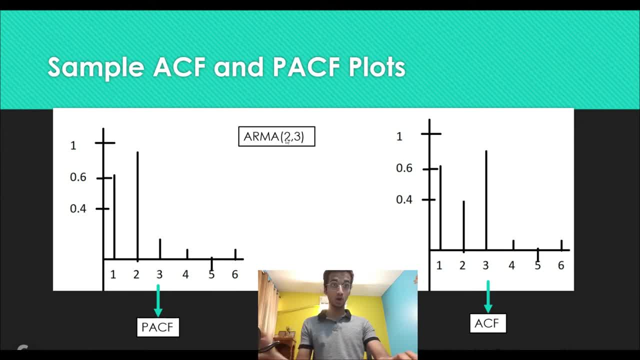 we have ARMA 2,3, and here 2 means second order auto regression. And as for the ACF plot, you can see that we getting significant values for one, two and three time periods back, which makes it a third order moving average model Right. The rest of the values for four. 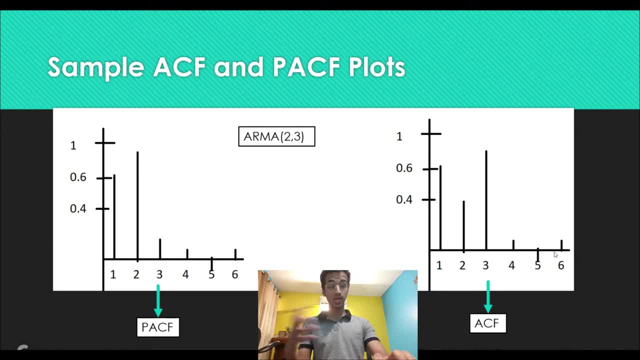 time period back. five time period back are very low. they are statistically insignificant and we don't consider that Right. In the ACF and ACF plot we can find the order of the auto regression and the moving average and combine them to get your ARMA model. So in this case we have ARMA model of 2,3 order. 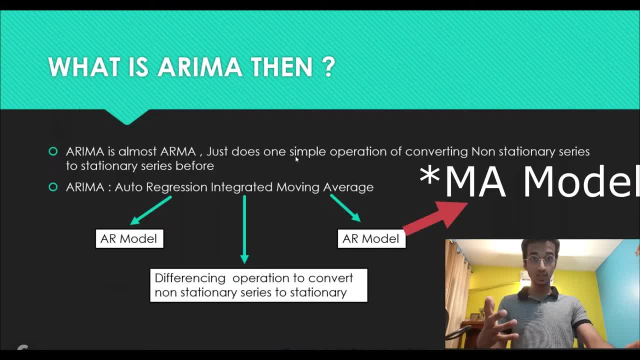 Right. So what is ARIMA? ARIMA is almost same as ARMA, with one key difference: that that in ARIMA model we convert a non stationary time series to a stationary time series and then proceed with the same thing. So don't get confused. I've explained. I explained. 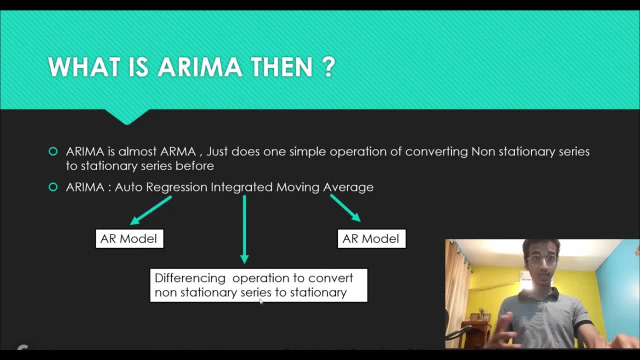 constantly of stationary and non stationary before as well. I'll explain it again, But let's look at the notation. So AR stands for auto regression, MA stands for moving average and A stands for integrated, which basically refers to a differencing operation which we have to. 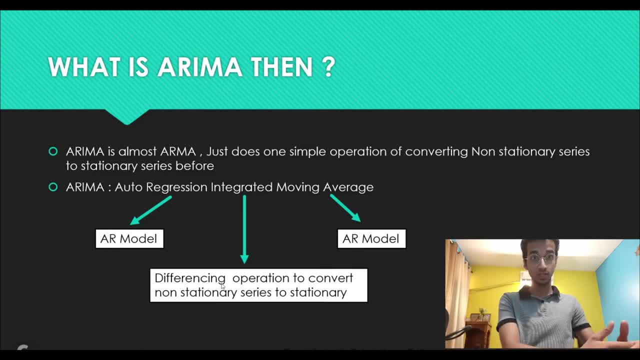 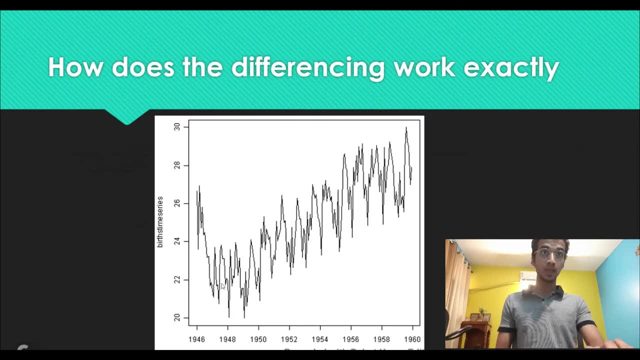 do to convert a non stationary time series to a stationary time series. So if you have not watched the previous videos on stationary time series, let me just give you a quick recap. Right, So let's say you have a time series like this, This type of time series, 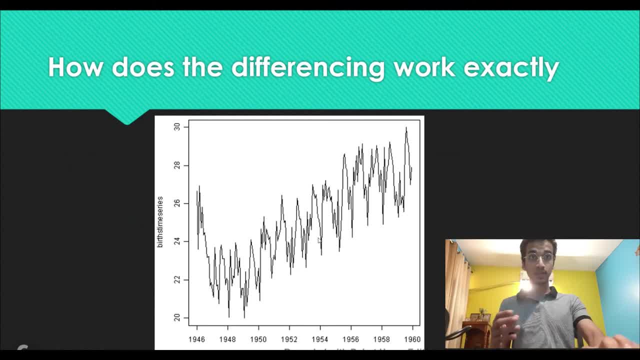 is called non stationary time series. This is a non stationary because the mean, the average value of the graph, is constantly increasing. Right You can see the values increasing from a low value to higher values. So a stationary time series basically has a constant mean, a constant variance, and it 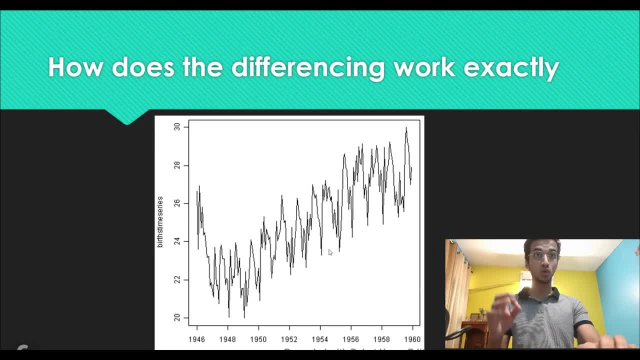 does not have a seasonality, So just focus that this does not have a constant mean right. So this means it's a non stationary time series and we cannot use that for modeling. So first step is using a differencing operation to convert that into stationary, which looks. 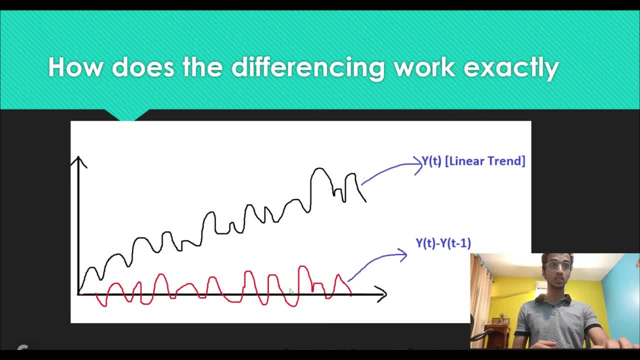 like this. Right, Let's say you have a graph like this, the black colored line which is a time series, And you can see the average constantly increasing. We have to convert that to a stationary time series by doing a differencing operation which looks like this: We're simply subtracting. 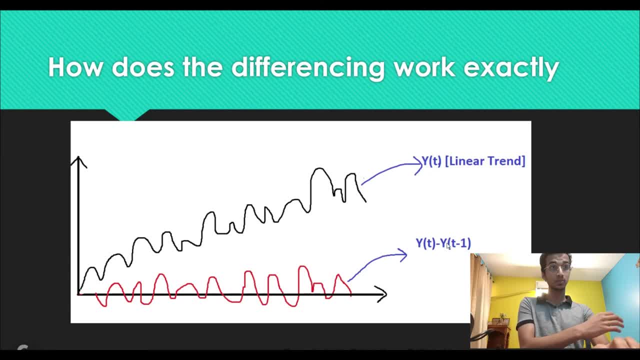 the values of the time series, the values in the previous time set, just basically y sub t minus y sub t minus one. And you can see, by doing that we eliminate the trend and we have somewhat of a stationary graph like, because we can see the mean is constantly. 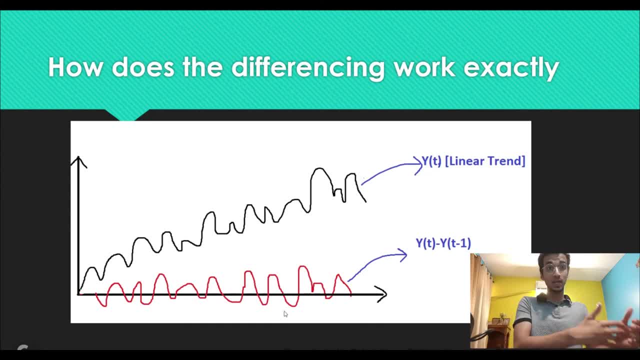 over here, Right? So depending on what kind of non stationary time series you have, you will have to do differencing operation. Since we're only subtracting the values in the previous time step. this call as first order difference. you might have to do second order differencing. 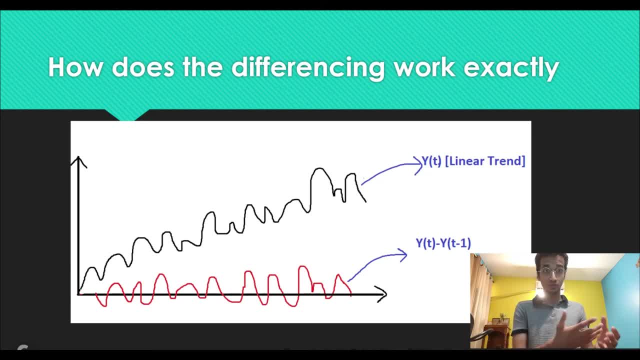 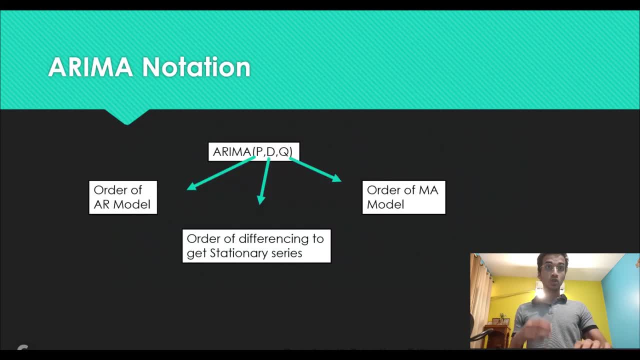 third order: differencing, to get a stationary graph. I've made an in depth video on my stationality video So I would recommend you watch that if you want to understand this in depth. So basically, you have the notation as P, comma D, comma Q for a Rima model, So it's same as. 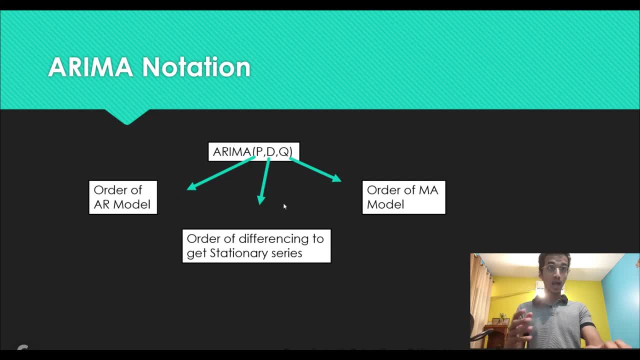 our map, P and Q stand for the order of air model and the order of ma model respectively, while as D stands for the order of differencing that you had to do to convert the non stationary graph into a stationary time series. So that was it for this video, guys. This was just 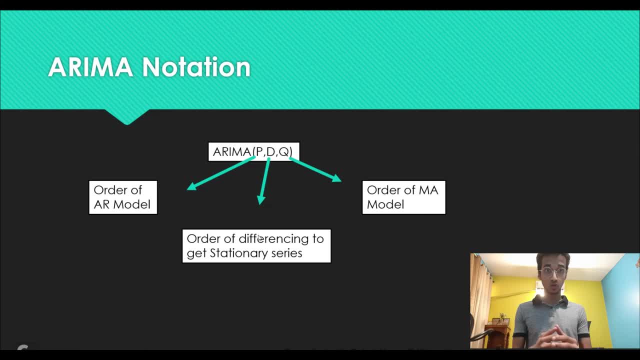 to clear the foundations of our Rima models for time series forecasting, which I'll show you how to implement that in Python. If you like this video, do like this video and subscribe to this channel. And yeah, thank you for watching.